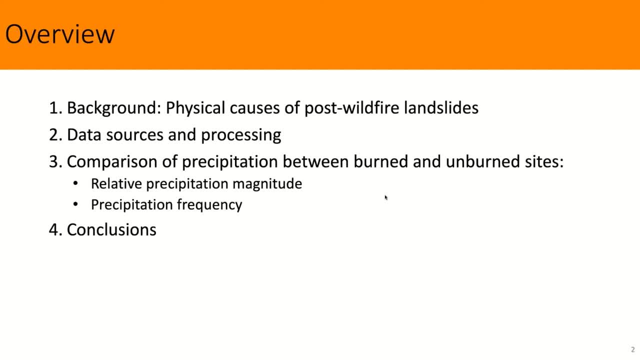 bit about why we think post-wildfire landslides are a special kind of thing, And then I'll talk about the data sources and the processing, And then, finally, I'm going to talk about how we're going to be comparing the precipitation between burned and unburned sites using a 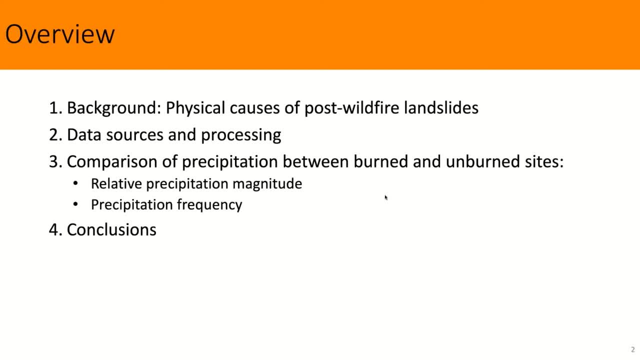 couple of different methods. I think each of them has something interesting and different to say about these precipitation triggers. So I'll first be looking just at the relative precipitation magnitude of these storms And then, secondly, I'll be looking at the frequency of precipitation. 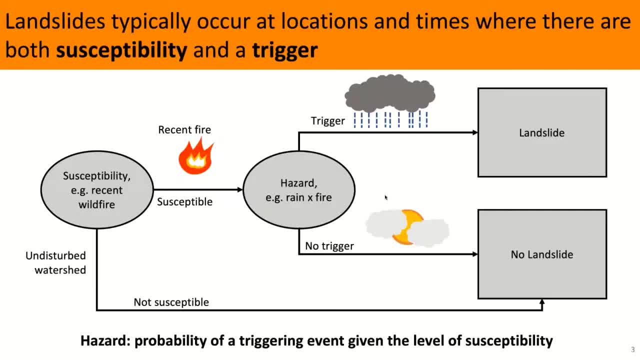 So landslides occur when there's both susceptibility and trigger. So what that means here is: the susceptibility in this case is something like a recent wildfire, And the fire makes it more likely, perhaps, that a landslide will happen, but it doesn't actually cause the landslide. 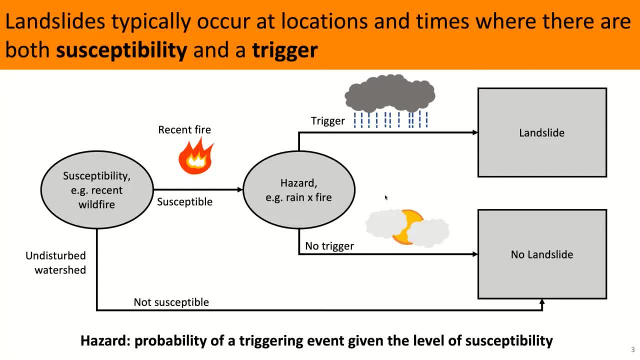 by itself And so for that we need a trigger, And so talking about hazard is kind of the probability of a triggering event at the given level of susceptibility. So whatever kind of volume of rainstorm in this case that might be might change based on the susceptibility And so 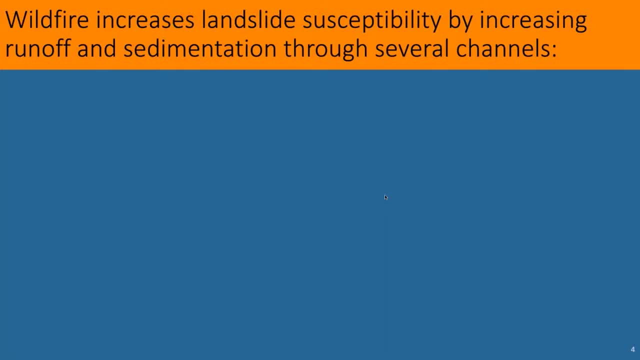 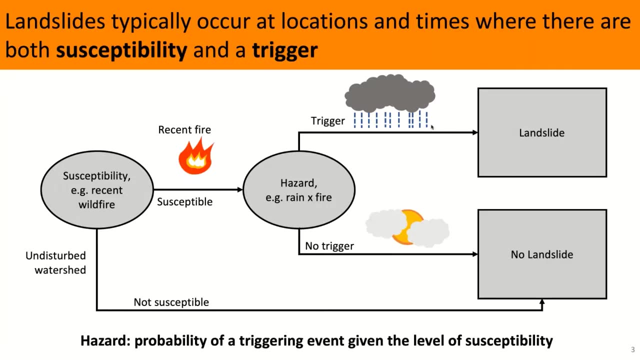 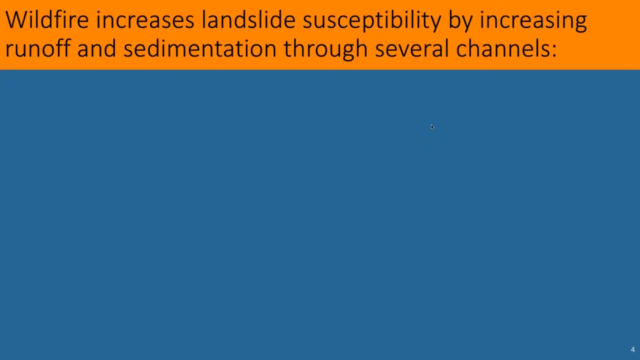 the hazard is really the combination of those two things. I'm sorry, my slide just moved by itself, Okay, but anyway, without both, without the trigger, we don't get the landslide, I guess is the point. And so a wildfire increases landslides, susceptibility in a couple of different sort of physical 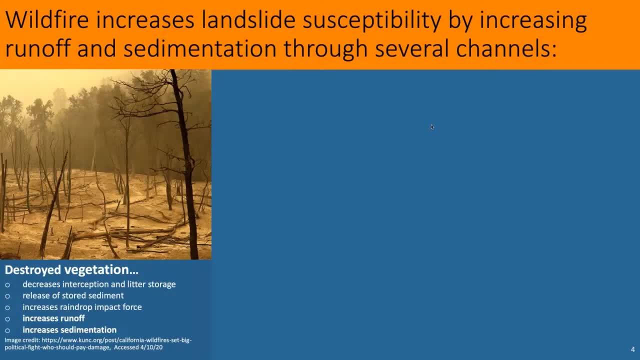 ways. So, first off, fire destroys vegetation. That's pretty much what this is all about. And then the third one than the last two. then the third one is when the landslide closes into the ground. I'm sorry, my slide just moved by itself. 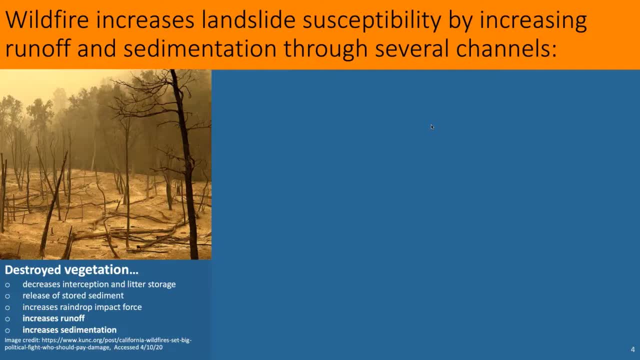 I'm sorry, I just moved by itself, But anyway, without both, without the, without the trigger, we don't get the landslide. I guess is the point: vegetation that decreases interception and litter storage and also releases sediment that's kind of stored behind trunks of vegetation and because there's no canopy it increases. 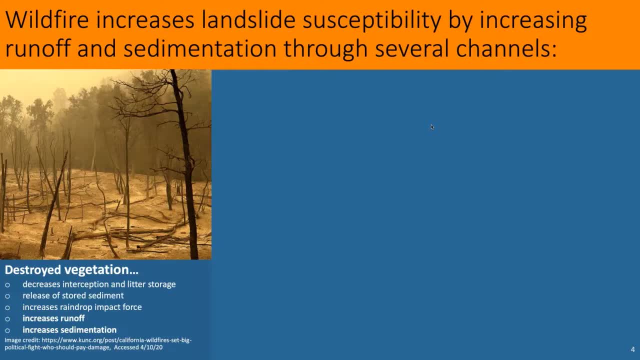 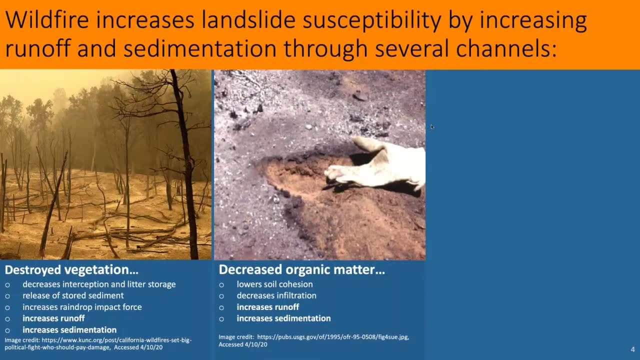 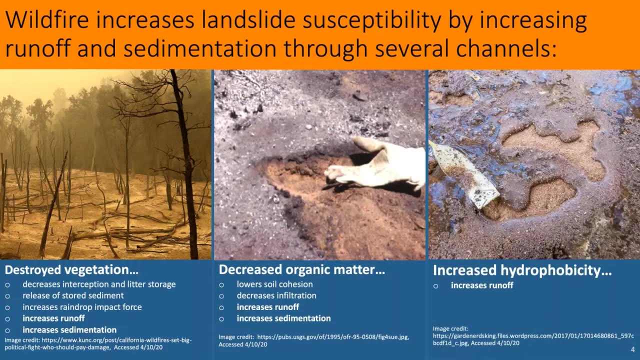 the raindrop impact force. In addition, fire can burn off some of the organic matter in soil, which lowers the soil cohesion and decreases infiltration at the same time. And then, finally, fire can create kind of a hydrophobic layer near the soil surface, which increases runoff because the water can't infiltrate, and what all of these things, all three of 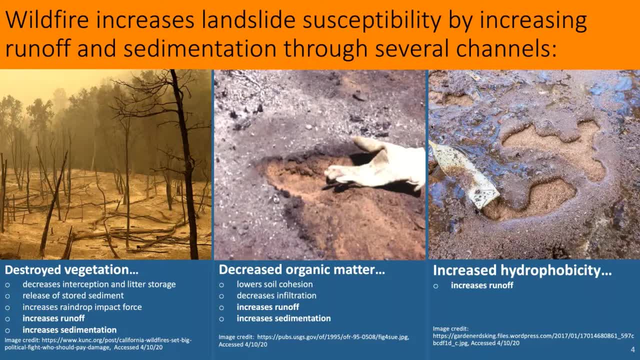 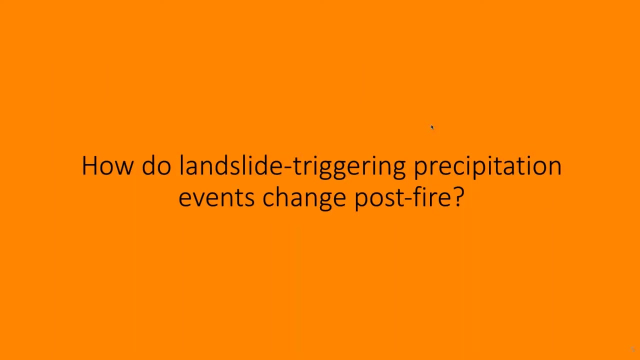 these things are increasing runoff and they're increasing sedimentation, and if there's enough of that going on, then that can get to the point Where it starts to create a debris flow or perhaps a slope failure. So what we want to know with this project is: how do landslide triggering precipitation 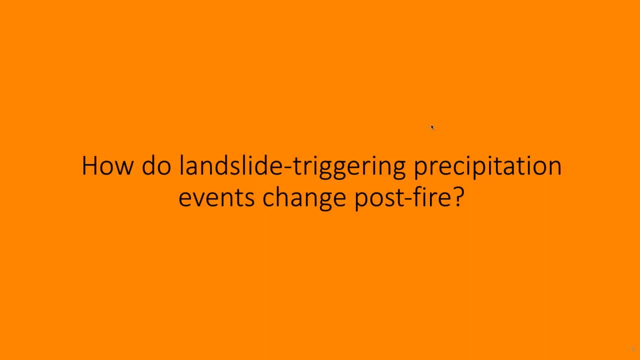 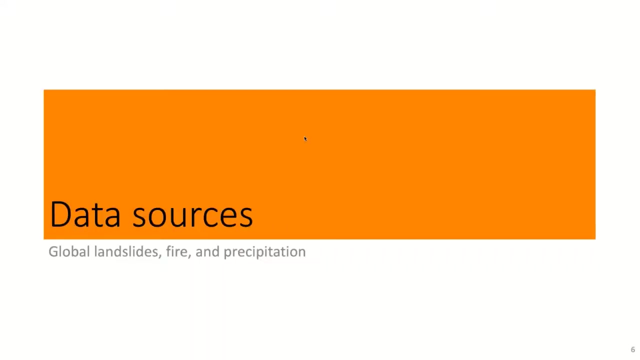 events change after a fire. So another way of putting that is like what kind of, what kind of magnitude or frequency of precipitation is required in order to- in order to get a landslide after a fire, as opposed to in an undisturbed watershed? And so next I'll be talking about the data sources, and so we've picked global data databases. 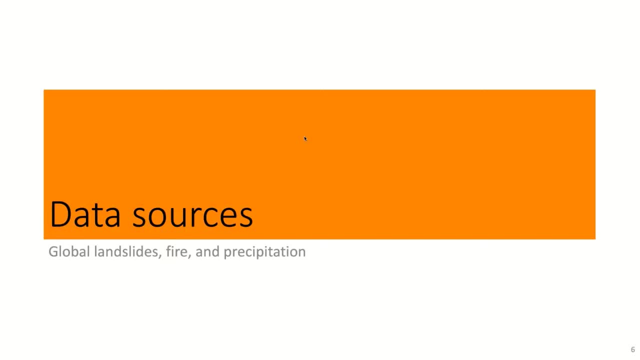 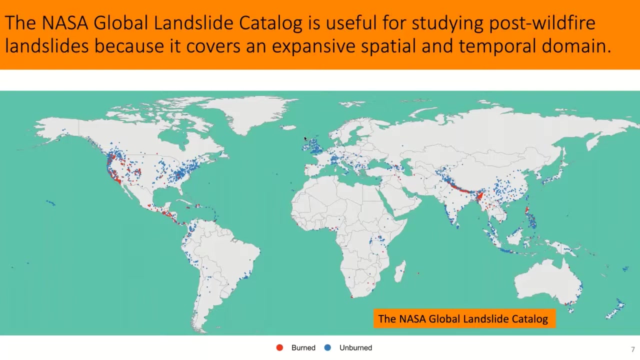 for landslides and fire and precipitation and, where possible, satellite based data sources. so the fire and precipitation. So that's the first one, Then our derived from satellite data. So first of all, the NASA global landslide catalog is the source of the landslides in. 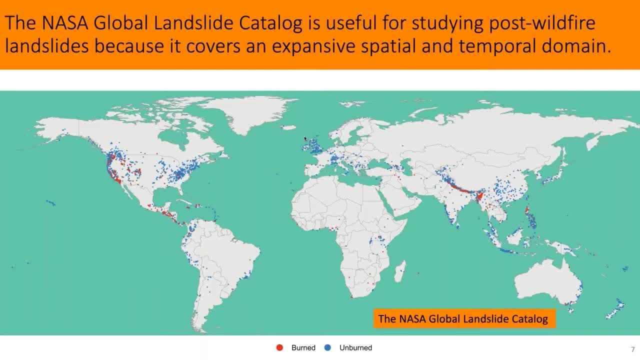 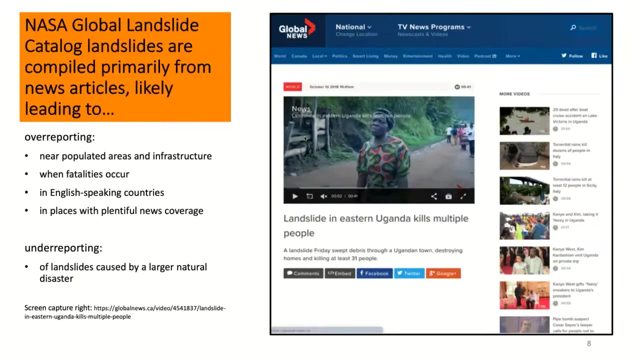 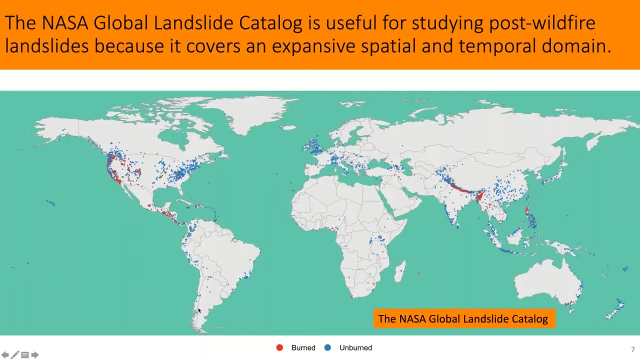 a study and it's useful for studying post-wildfire landslides because it covers just an expansive spatial and temporal domain. This is a little unusual in landslide inventories: they tend to be fairly localized, both spatially and then also temporally, Because there will be perhaps one large triggering event, that that that causes a number of landslides. 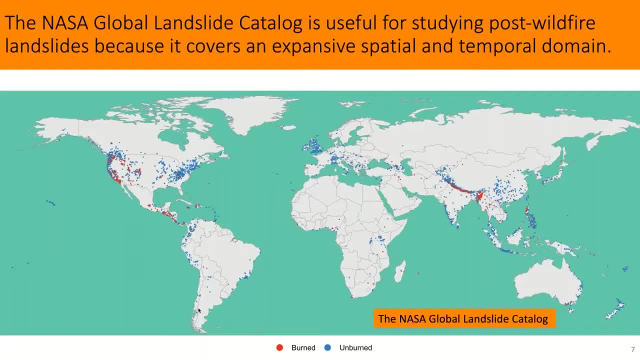 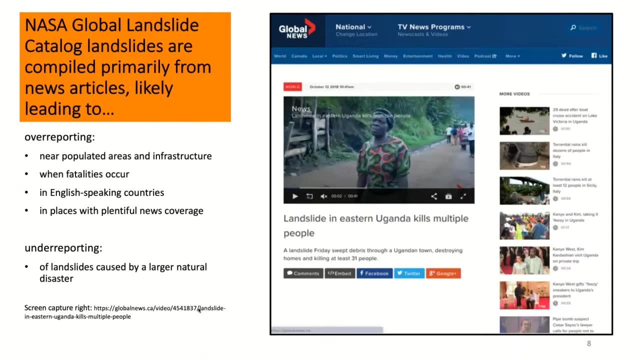 and then someone will go out and do a survey, but that that only tells you about that one snapshot in time. The disadvantage of the NASA global landslide catalog is that the landslides are compiled primarily from news articles, and so that means we get a lot of landslides that are 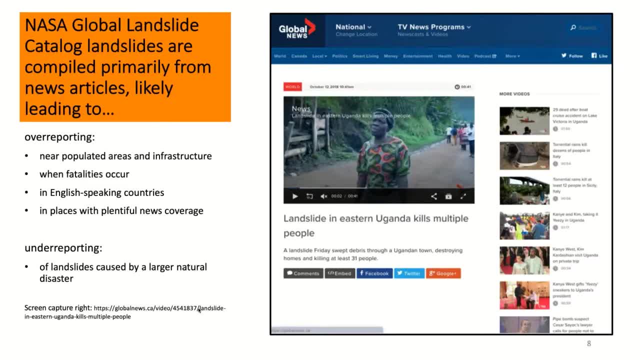 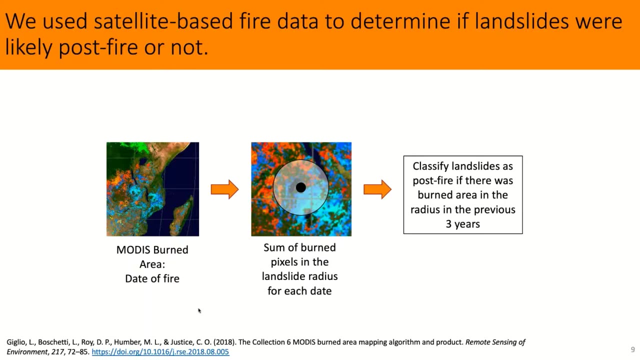 near populated areas in English-speaking countries with plentiful news coverage, and also means that we kind of miss landslides that are caused by a larger natural disaster because the coverage gets eclipsed. Moving on to the fire data, This is the. The data is derived from MODIS burned area data set, which is essentially the date of 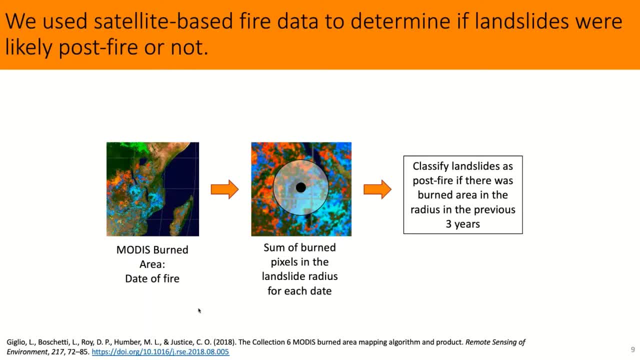 fire for, for across the grid, and so like. the similar colors in in this diagram would indicate a similar fire event or the same fire event. So then, what we do is we just check, within the landslide radius for each date, if there's been any fire and add up that, add up that fraction of the area that has been burned. 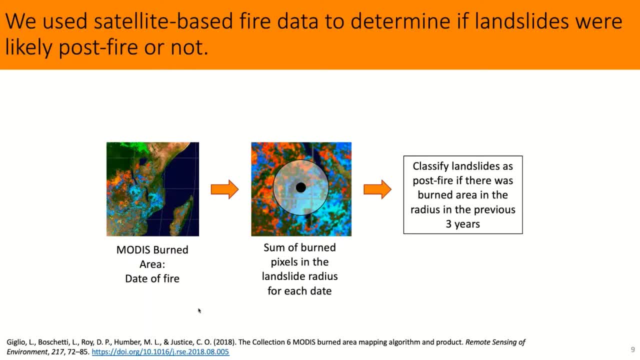 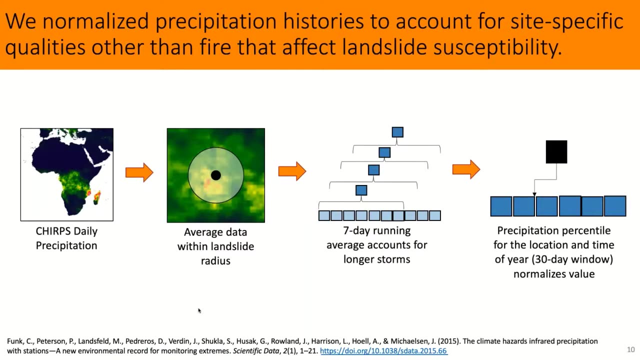 within the previous three years- Sorry, the three years prior to the landslide. and then we classify landslides as post fire, if there's any burned area in there at all in those previous three years and the precipitation is is similar process, but we did a couple of other. 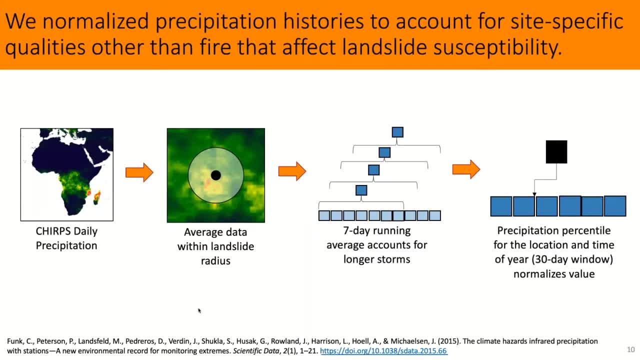 A couple of other things in order to try to account for some of some of the the things that we observed happening with just sort of the raw precipitation data, and start off with the church's daily precipitation data set And then again average the data within the landslide radius. 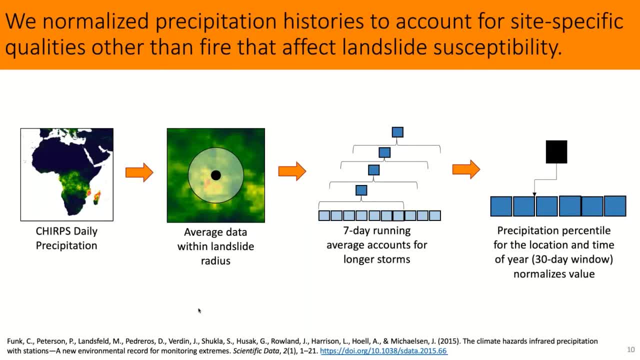 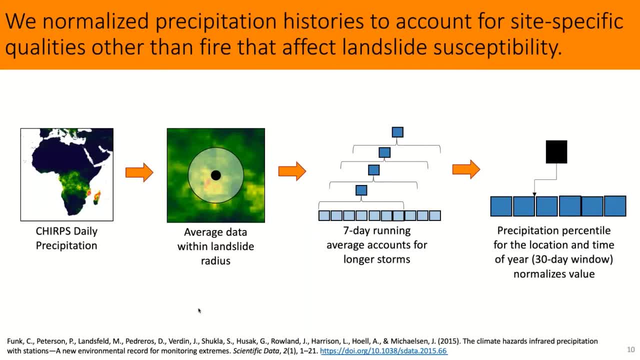 of pull in those longer precipitation events as a single data point. And then, finally, finally, we We tried to normalize the data based off of the location and the time of year, by which I mean, like a 30-day window around the event. 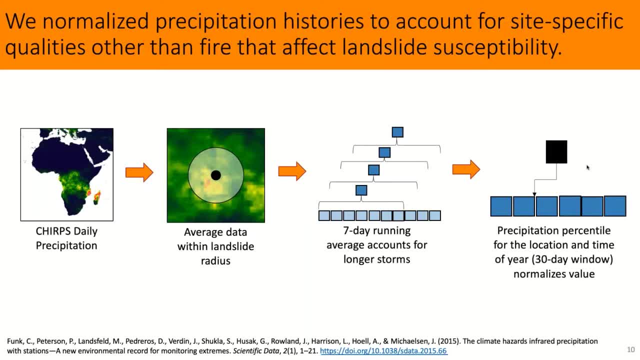 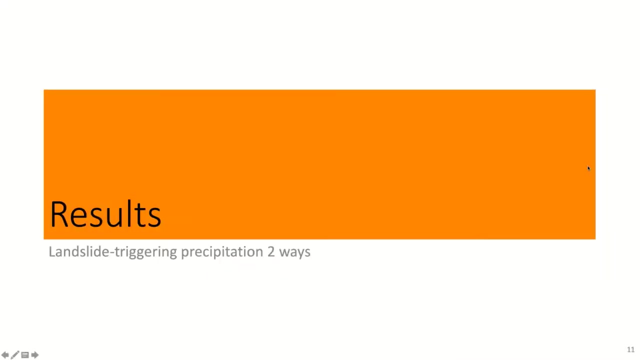 And so we've pulled from the TURPS record, which is about 40 years, and that 30-day window around the landslide day of the year, all of that data, and then calculated the percentile of the precipitation that we actually encountered. 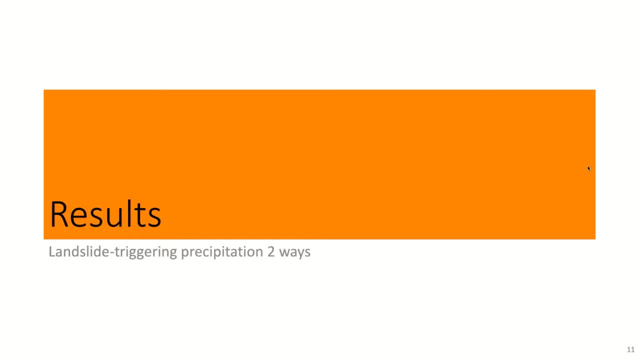 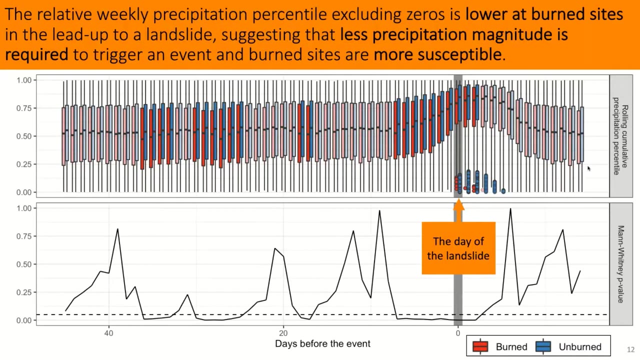 So, moving on to the results, I'm going to start out with the precipitation magnitude. So this is the precipitation values that I was talking about in the previous slide, But I have excluded all of the zero precipitation days, And the reason for that is because the magnitudes are normalized by the site and the time of 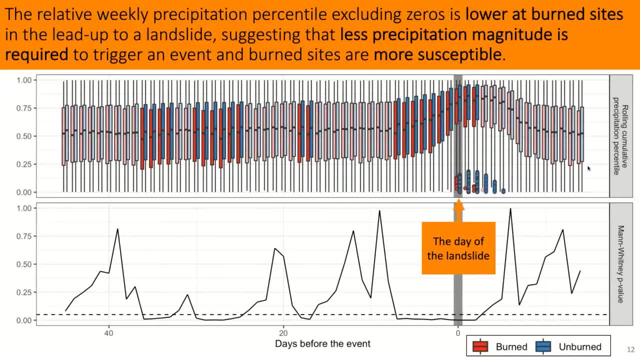 year, but the precipitation frequency is not normalized, And so it was difficult to tell what was really going on With these data, with the zeros in there, because there were some persistent differences between the burned sites and the unburned sites. So the day of the landslide is indicated by that big orange arrow. 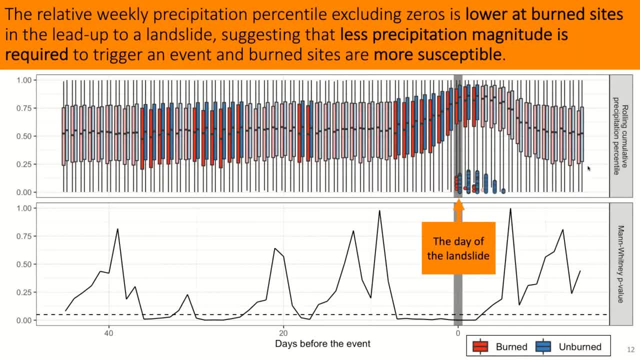 And so this time axis is not a, Is not Like any particular Date. It's all relative to when the landslide happened at a particular site, And these box plots are showing the precipitation at all of the landslide sites, but grouped by the fire history. 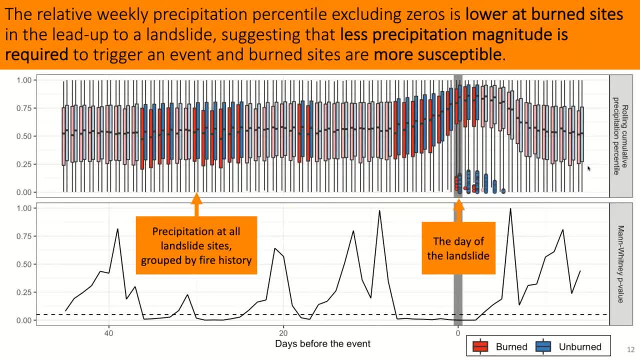 So those red box plots are the burned sites and the blue box plots are the unburned sites, And the first thing that you can see looking at this plot is that the precipitation is increasing as the landslide approaches. And that's not too surprising, because they're rainfall triggered landslides and we would 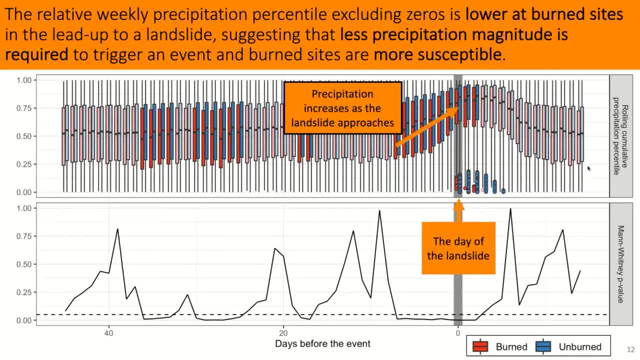 expect to see some rain happening, But what we also did was to compare the two distributions, the burned and the unburned at each day, to see if there was any statistically significant difference. We used a Mann-Whitney test for that. 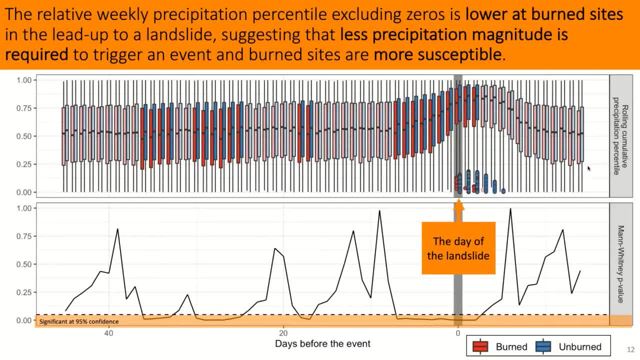 And so, looking down at the lower panel, you can see that there's a region around when the landslide happened where there is a sort of consistent, statistically significant difference And that That is indicating that there's less precipitation at the burned sites, And the implication of that for our landslide hazard is that less precipitation magnitude. 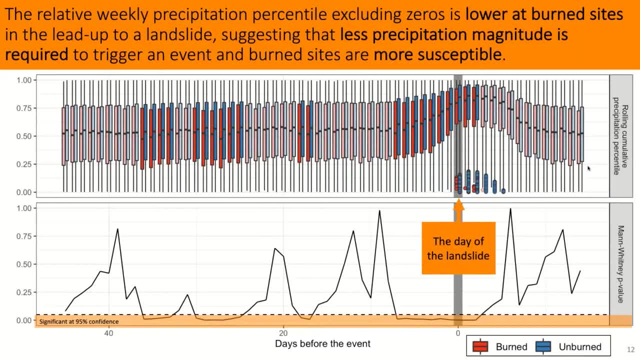 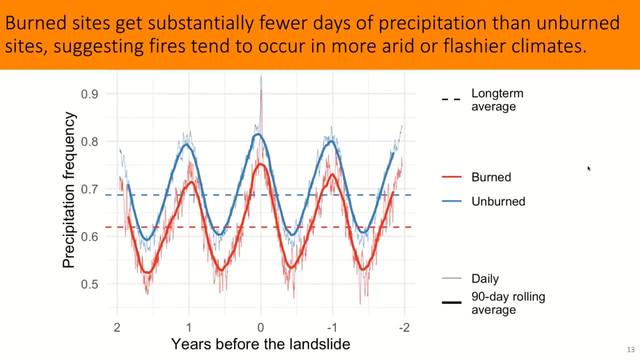 is required in order to trigger a landslide at the burned sites, and that in turn implies that, Okay, That the burned sites are more susceptible to landslides. Moving on to the second part of the results, here with the precipitation frequency, So I've just plotted the precipitation frequency here and, as I mentioned, these aren't normalized. 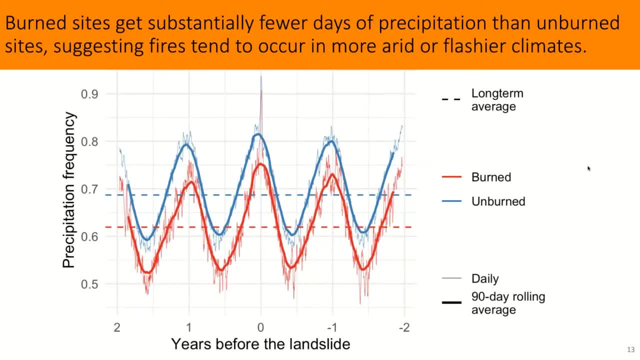 by the site And as a result of that we see a constant sort of a constant difference in frequency throughout the entire record. Those dotted lines are showing the long-term average And so that It's a little hard to see what's going on as far as our landslides, susceptibility, but 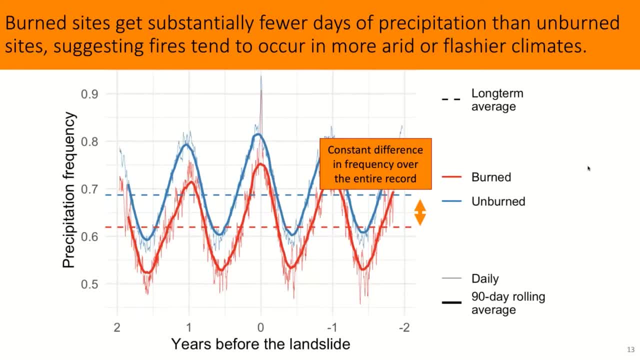 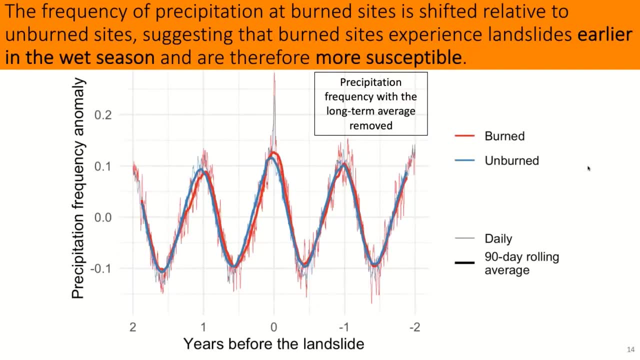 it does suggest something about the fires that they're occurring in perhaps more arid or in kind of flashier climates. Okay, But what I've done for this plot is removed that long-term average And so you can see these curves are much more similar to each other, but also that the red 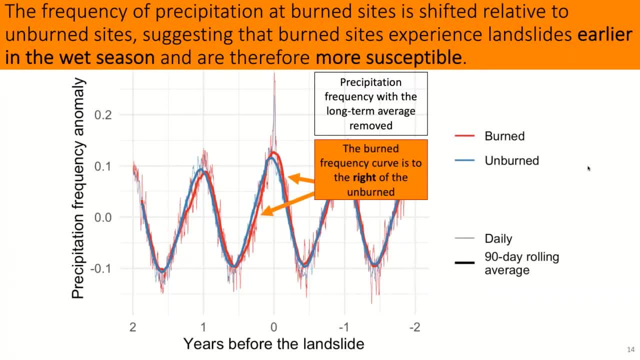 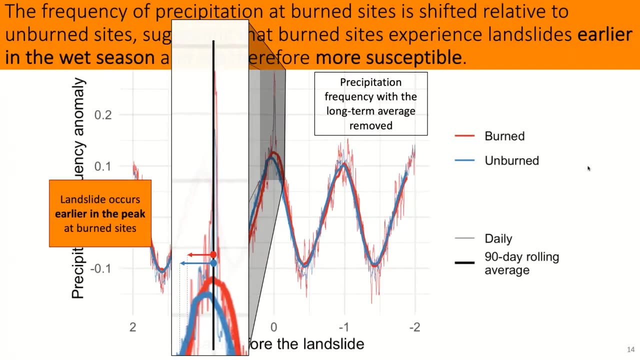 curve is consistently shifted as compared to the blue curve, So it's always to the right, especially in that year of the landslide. Okay, And so what that means is that the landslide is occurring earlier in the sort of wet season peak at burned sites. 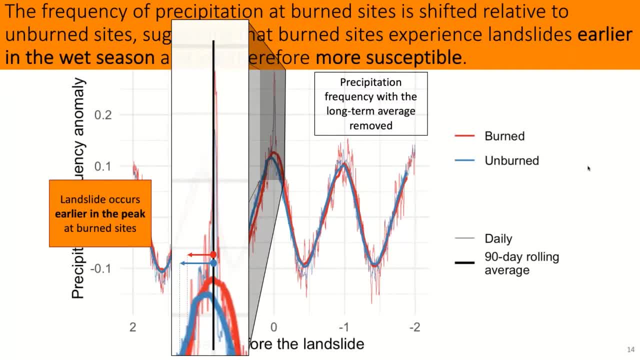 You can see the red arrow there, which is going to the edge of the peak from the landslide, is shorter than the blue arrow. Okay, Okay, Okay. So we think means that the burned sites are more susceptible to landslides because that it doesn't take as much of that wet season precipitation building up soil moisture in.